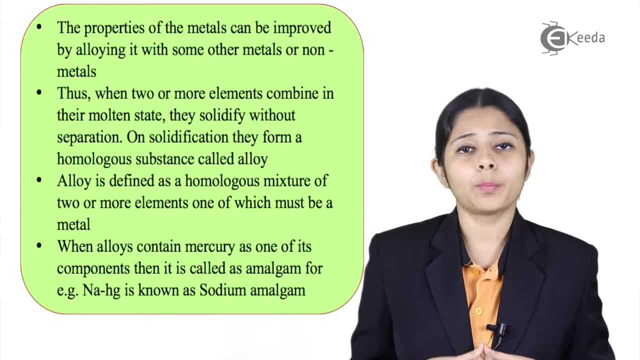 into something or the other to make them to use. The properties of metals are such that they are very ductile and malleable. Metals inherently are soft. When I say soft, they cannot resist wear and tear, they cannot resist a lot of resistance and they break off. So 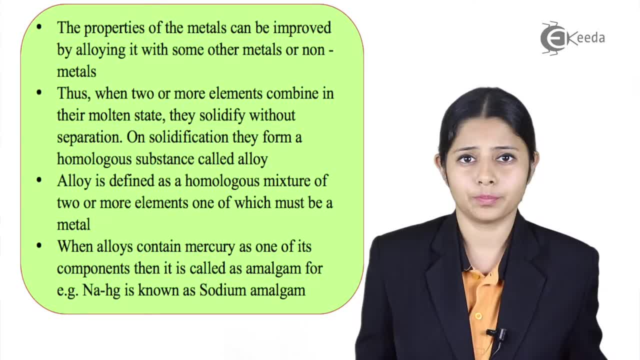 to make them tough, to make them strong, we need to alloy them. What is basically alloying? Alloying is basically getting two elements in their molten state, one of which, of course, should be a metal, and then combining them together and letting them to solidify. If 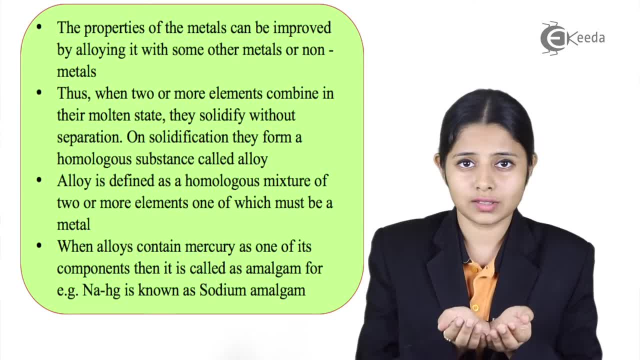 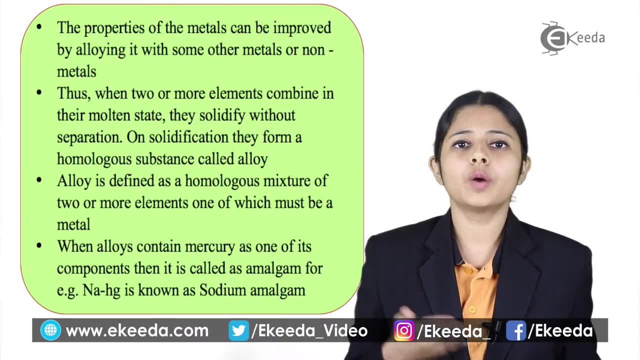 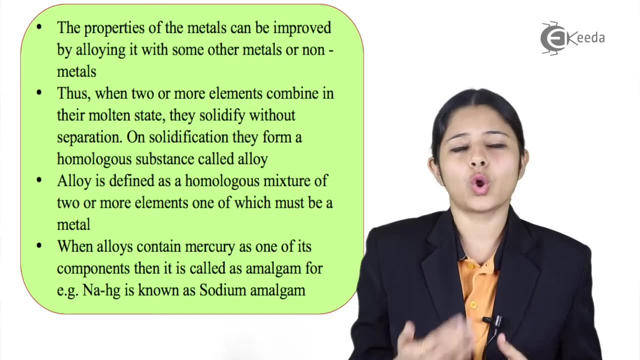 they solidify without separation into one homologous substance. that substance is known as alloy. Alloy is defined as a homologous mixture of two or more elements, out of which one has to be a metal. Alloying helps to improve the properties of a metal in a lot of ways. 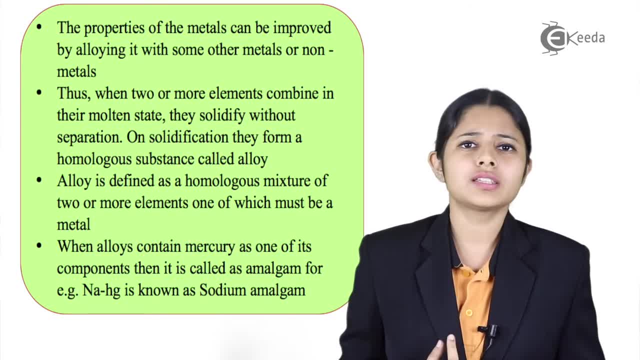 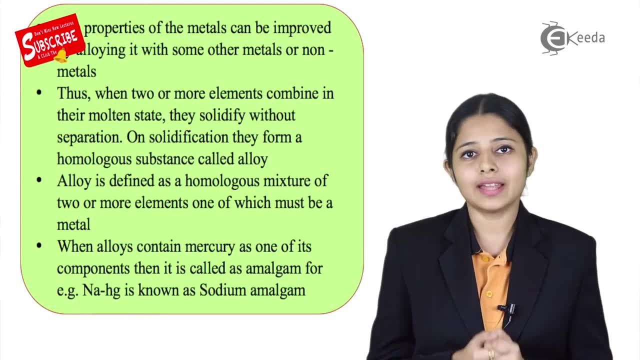 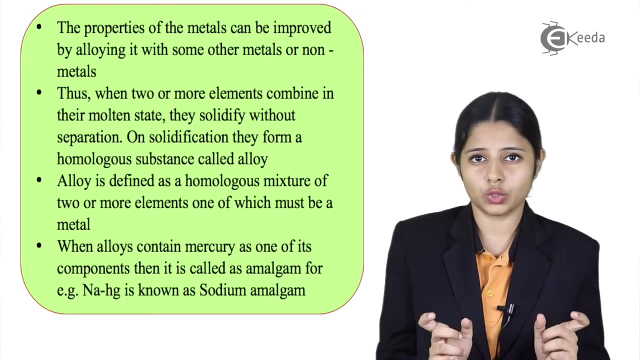 The metals become tough, they become strong, they resist a lot of wear and tear and they are much easier to use. If a molten metal is mixed with mercury, then that alloy is known as amalgam. For example, Na and Hg, where Na is sodium and Hg is mercury. this 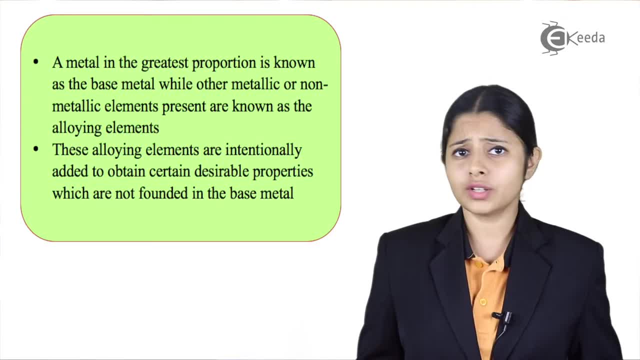 is known as a sodium amalgam For making alloys. it is not necessary that we have to add in something which is metallic to the base metal. We can add anything which is either metallic or non-metallic to the base metal. We can add anything which is either metallic or non-metallic. 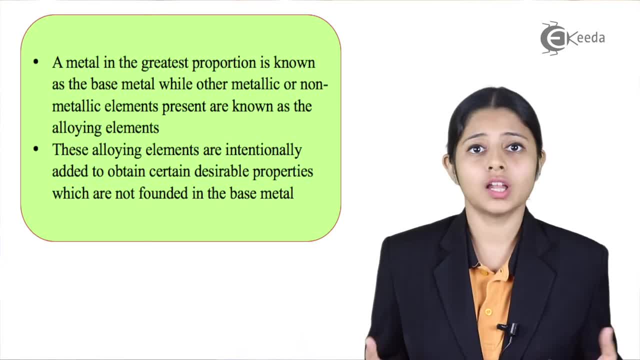 to the base metal, But a metallic-non-metallic combination- that is the alloy that has been formed, should make sure and ensure that the properties of metals have been increased and that metal is of great usage. now. In an alloy, the metal in the greatest proportion is known. 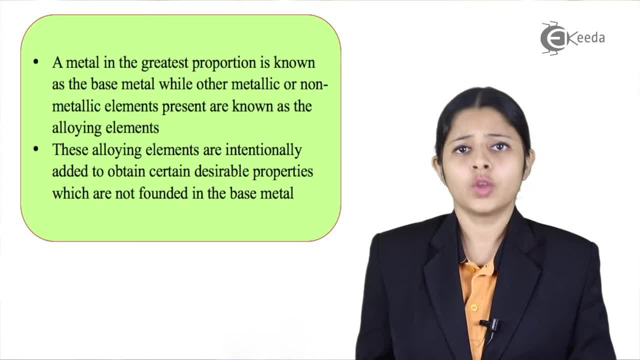 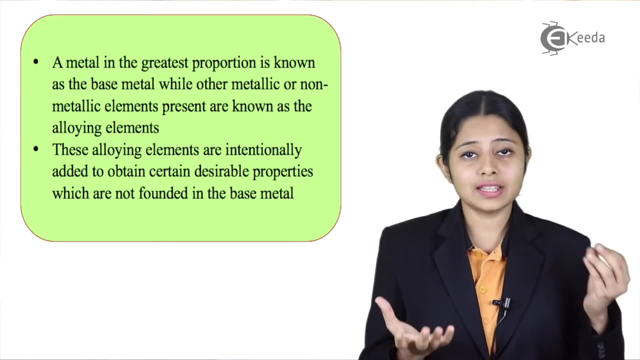 as the base metal and anything we add on top of it, whether it is a metal or a non-metal, it is known as the alloying element. The alloying element is intentionally added to the base metal to get the desirable properties of the metal. 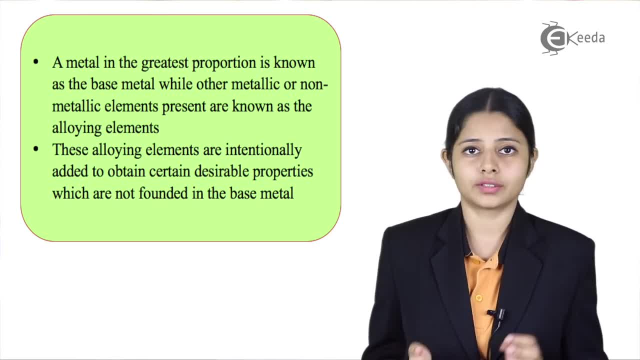 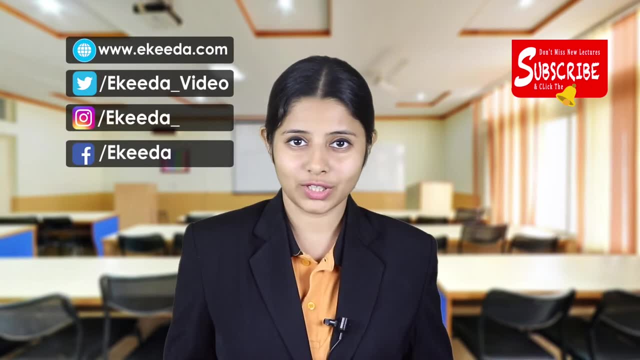 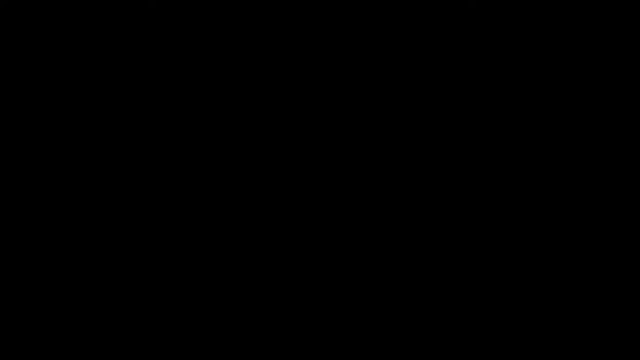 So in this video there was introduction of alloys and why alloys are very necessary. Thank you so much for watching this video. Stay tuned to eKeda and subscribe to eKeda. Thank you for watching this video. Stay tuned to eKeda.